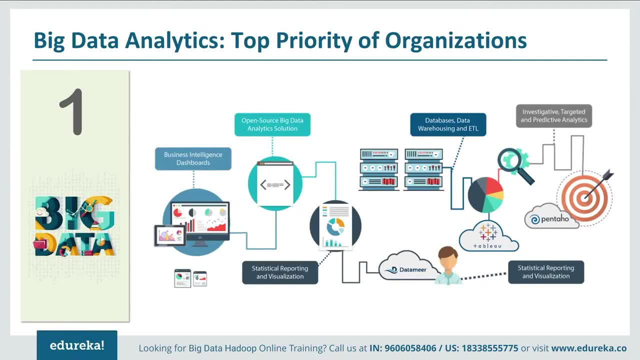 years. In fact, big data has been adopted by vast number of organizations belonging to various domains, And, by examining large data sets using big data tools like Hadoop and Spark, they are able to identify hidden patterns, to find unknown correlations, market trends, customer preferences and other useful business information. And let me tell you. 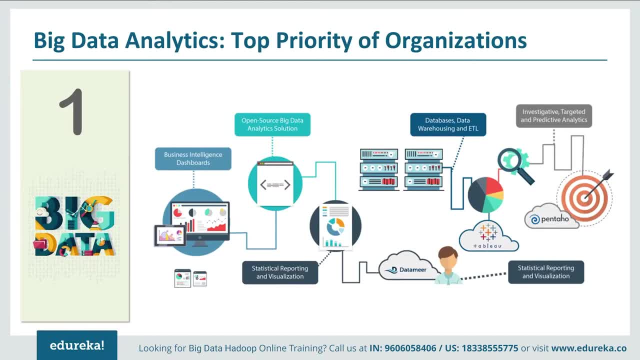 that in an article in Forbes, it was published that Big data adoption has reached up to 53% in 2017, from 17% in 2015, with telecom and financial services leading early adopters, And the primary goal of big data analytics is to help companies. 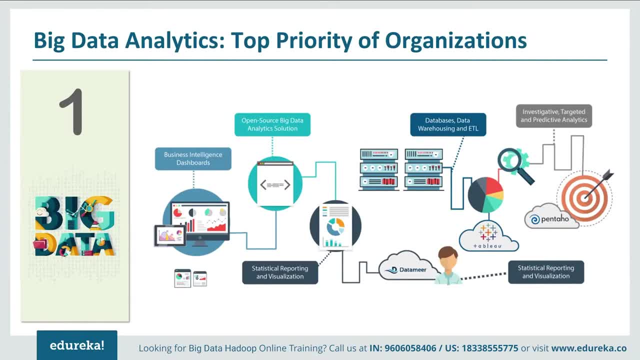 make better and effective business strategies by analyzing large data volumes. The data sources include web server logs, internet clickstream data, social media content and activity reports, Text from customer emails, phone call details and machine data captured by sensors and connected to the internet of things- IoT, as we call it. 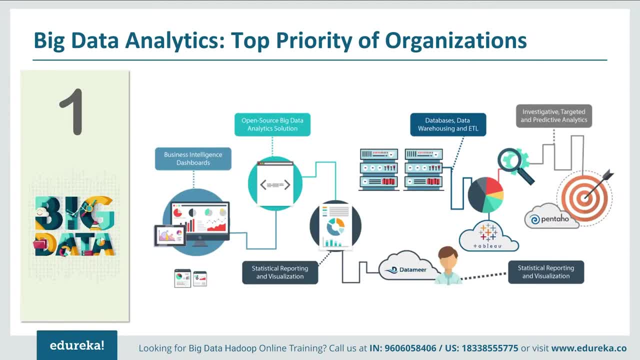 Big data analytics can lead to more effective marketing, new revenue opportunities, better customer services, improved operational efficiency, competitive advantages over rival organizations and other business benefits, And that is why it is so much widely used, And IDC says that the commercial purchases of big data and business analytics related hardware, software and 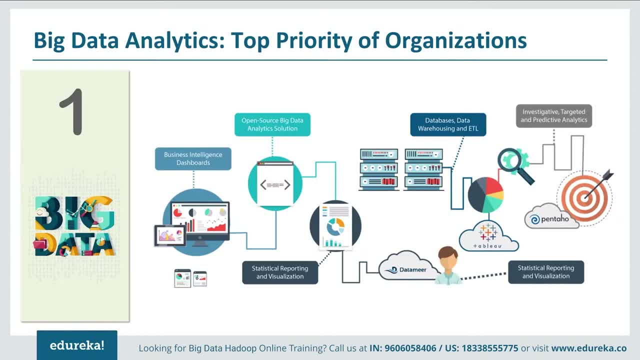 services are expected to maintain a compound annual growth rate of 11.9% through 2020, when revenues will be more than $210 billion. And that is huge. And the image here clearly shows the tremendous increase in unstructured data. like images, 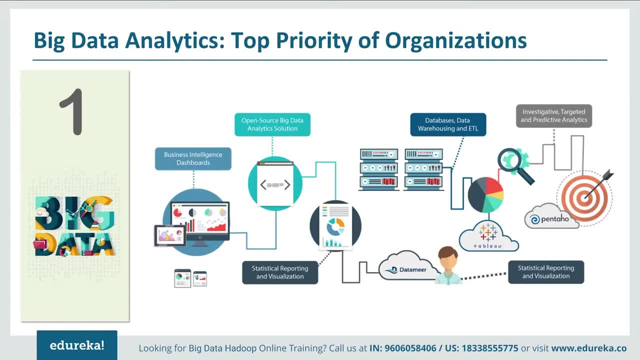 mails, audio, etc. Which can only be analyzed by adopting big data technologies like Hadoop, Spark, Hive and others. This has led to a serious amount of skill gap with respect to available big data professionals in the current IT market, And hence it is not at all surprising to see a lot of buzz. 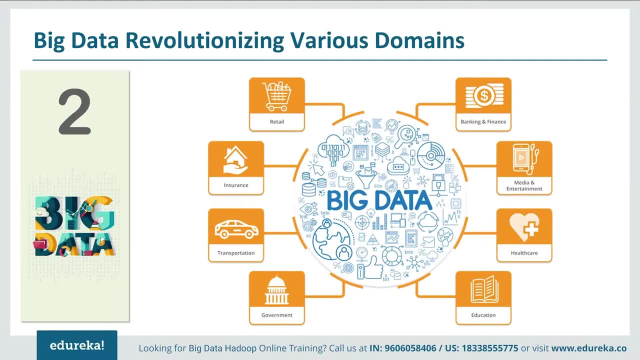 in the market to learn Hadoop. Reason number two: Big data is revolutionizing various domains. Now, big data is not leaving any stone unturned nowadays. What I mean by this is that big data is present in each and every domain, Allowing organizations. 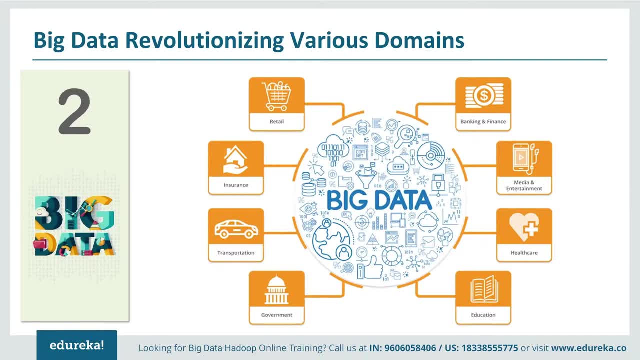 to leverage its capability for improving their business values. The most common domain which are rigorously using big data and Hadoop are healthcare, retail government, banking, media and entertainment, transportation, natural resources and so on, as shown in the image over here. 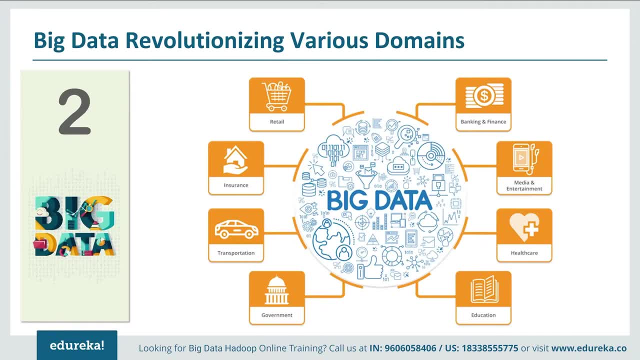 Well, to be honest, it is not only limited up to these domains. It is also limited to the domains mentioned here. Big data is spreading even more across different domains. As the technology is evolving, the data is increasing and hence big data is getting adopted across. 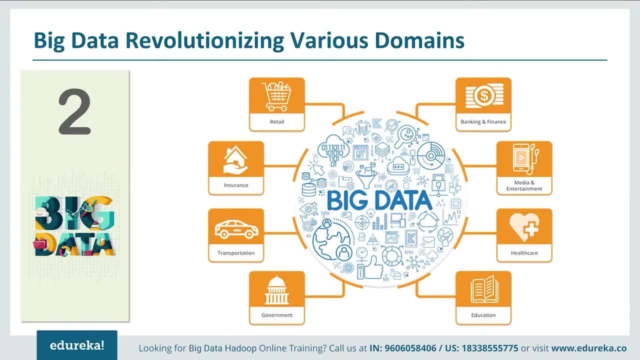 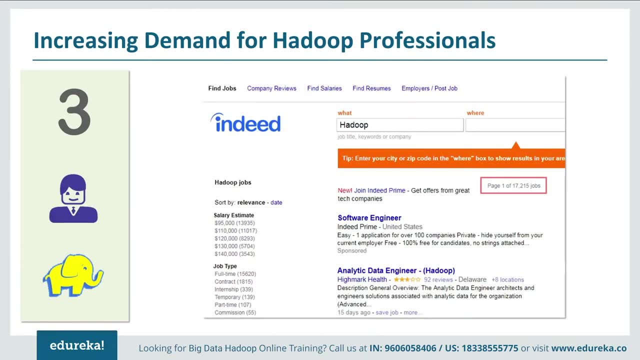 a wide range of domains. Hence you can build your career in any of these domains by learning Hadoop. Reason number three: Increasing demand for Hadoop professionals. The demand of Hadoop can be directly attributed with the fact that this is one of the most 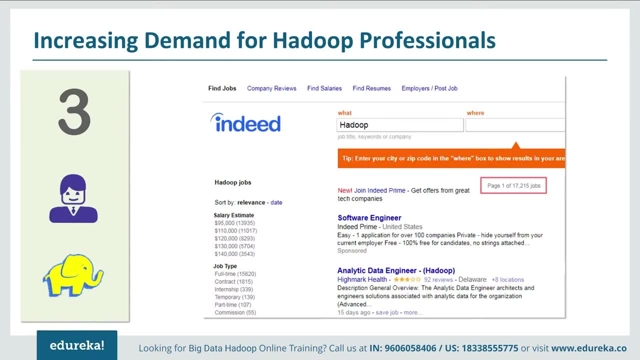 prominent technologies in the world. This is the reason why Hadoop has become so popular. It is a technology that can handle big data and is quite cost-effective and scalable. With the swift increase in big data sources and amount of data, Hadoop has become more. 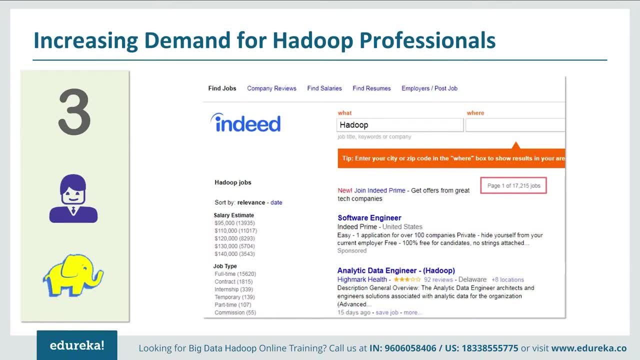 of a foundation for other big data technologies evolving around it, such as Spark, Hive, etc. And this is generating a large number of Hadoop jobs at a very steep rate. You can check out different job portals like Indeedcom, Knockread Times, Job, etc. and you will see the demand. 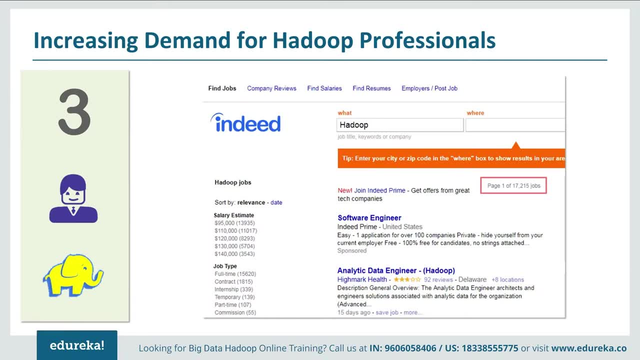 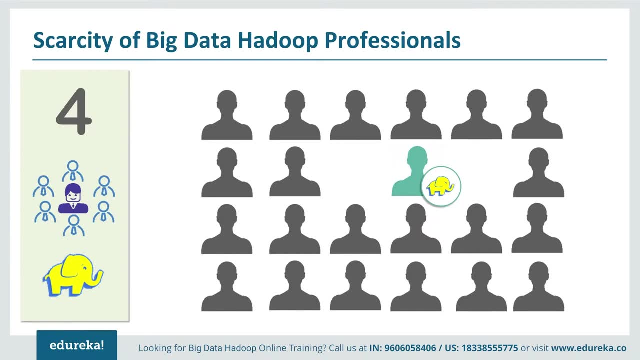 of Hadoop professionals when you browse through the Hadoop website. Thank you. Reason number four: Scarcity of big data- Hadoop professionals. Now, the demand must be more, but the supply is quite less, And as we discussed Hadoop, 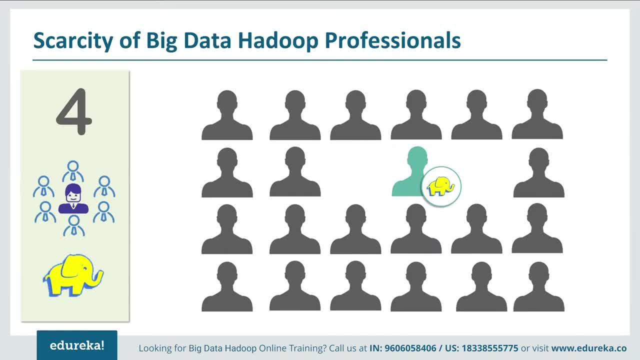 job opportunities are growing at a high pace, But most of these job roles are still vacant due to a huge skill gap that is still persisting in the market, And such scarcity of proper skillset for big data and Hadoop technology has created a vast 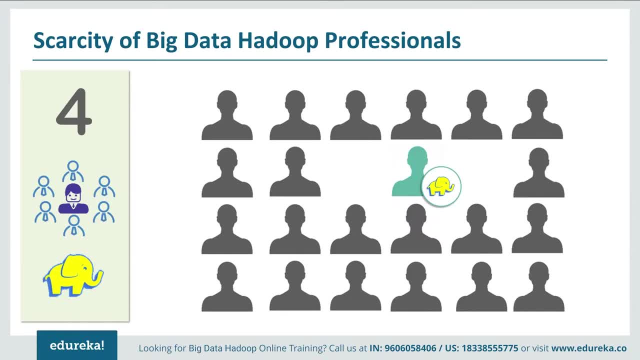 gap between supply and demand, And hence now it is the right time for you to step ahead and start your journey towards building a bright career in big data and Hadoop. In fact, the famous saying now or never- this is an apt description that explains the 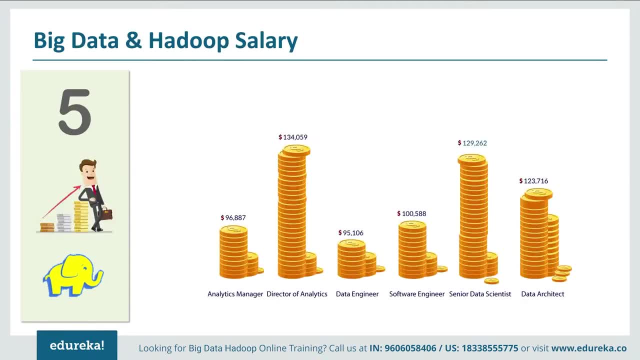 current opportunities in the big data and Hadoop market. Reason number five: Big data and Hadoop salary. This, in fact, is quite rewarding. One of the captivating reasons to learn Hadoop is the fat paycheck that you are going to make. This is the reason that you are going to have to. 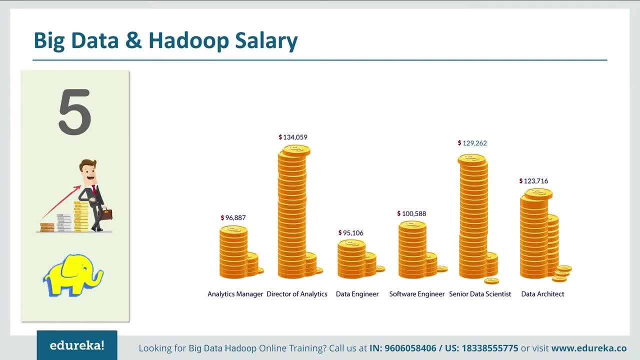 invest in Hadoop. The scarcity of Hadoop professionals is one of the major reasons behind their high salary And, according to Payscalecom, the salary of a Hadoop professional varies from $93,000 to $127,000 per annum, based on different job roles. You can see the different job roles. 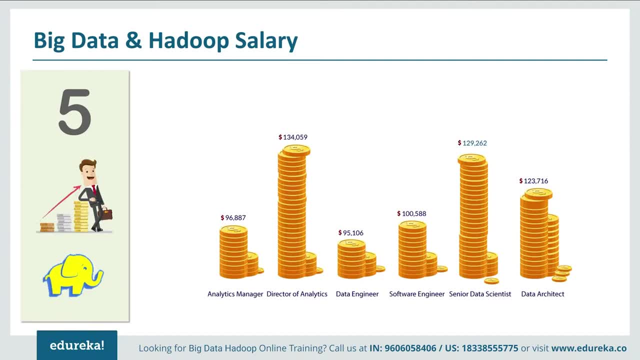 and their annual salaries over here, But of course it can vary according to the organization that you are joined in and also with the experience that you are going to have. You can also see the different job roles and their annual salaries over here, But of course it can vary according. 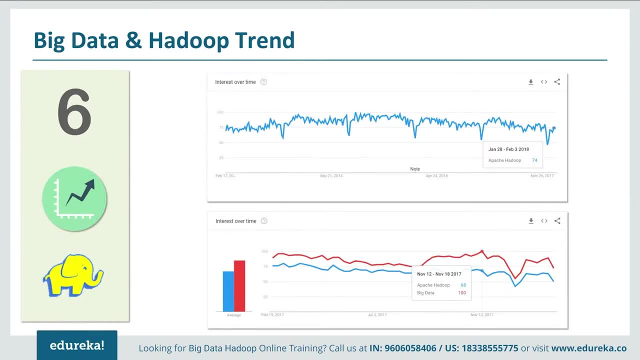 to the organization that you are joined in and also with the experience that you are going to have. Reason number six: The Big Data and Hadoop trend. and as per Google trends, Hadoop has a stable graph in the past five years, And one more interesting thing to notice here is that the trend of big data and Hadoop are 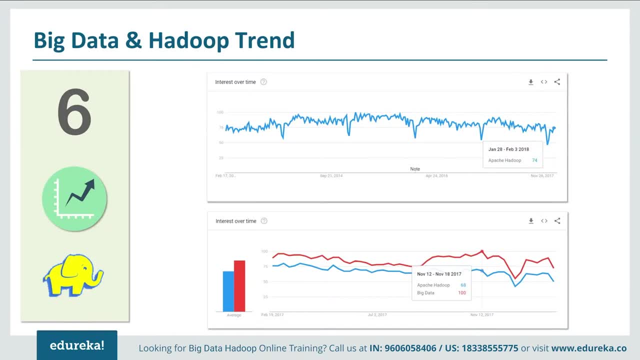 tightly coupled with each other. You can see over here that they go hand-in-hand and have a direct correlation. Big data is something which talks about the, a problem that is associated with storage, curation, processing and analyzing of the huge amount of data, and hence it is quite evident that all of the companies need to tackle the big data. 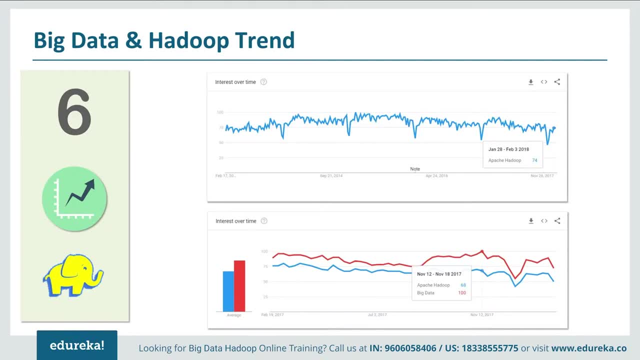 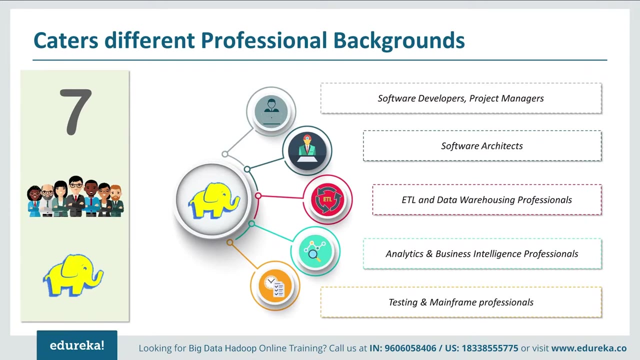 problem one way or another for making better business decisions, and hence one can clearly deduce that big data and Hadoop has a promising future and is not something that is going to vanish into thin air, at least for the next 20 years. Reason number seven: it caters different. 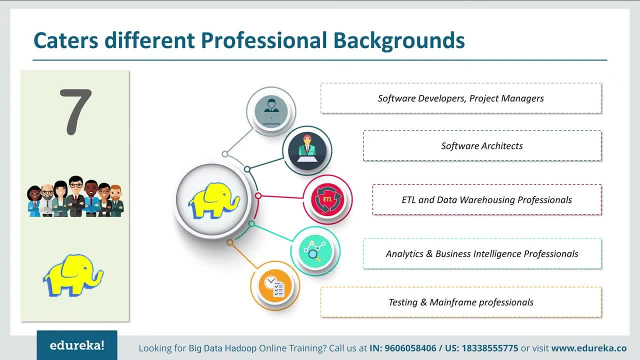 professional backgrounds. Hadoop ecosystem has various tools which can be leveraged by professionals from different backgrounds. If you are from programming background, you can write MapReduce codes in different languages like Java, Python, etc. If you're exposed to scripting language, Apache Pig is the best fit for you, and if you're comfortable with the 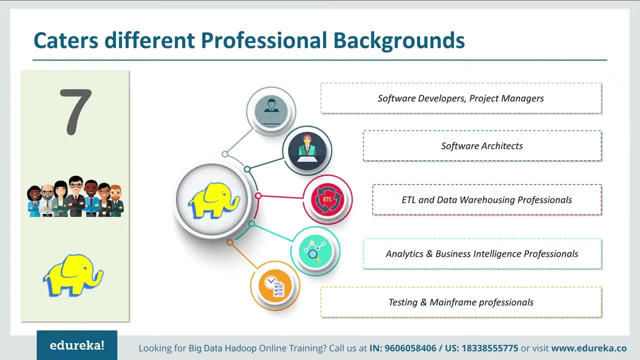 SQL. then you can also go ahead with Apache Hive or Apache Drill. The market of big data analytics is growing across the world and its strong growth pattern translates into great opportunity for IT professionals. It is suited for developers, project managers, software architects. 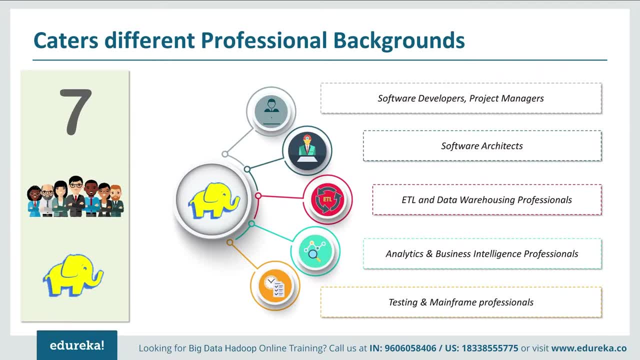 ETL and data warehousing professionals, analytics and business intelligence professionals, and also for testing and mainframe professionals. It is suited for developers, project managers, software architects, ETL and data warehousing professionals. It is also recommendable for freshers who are going to start a fresh career. 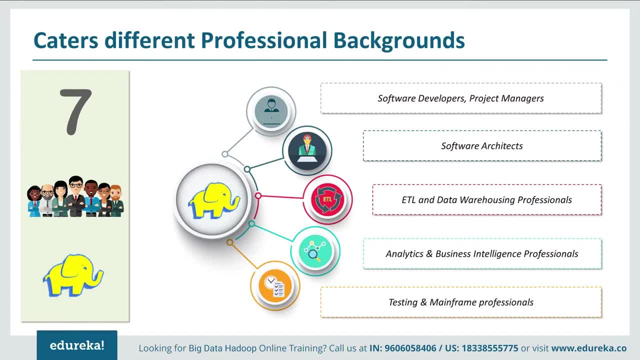 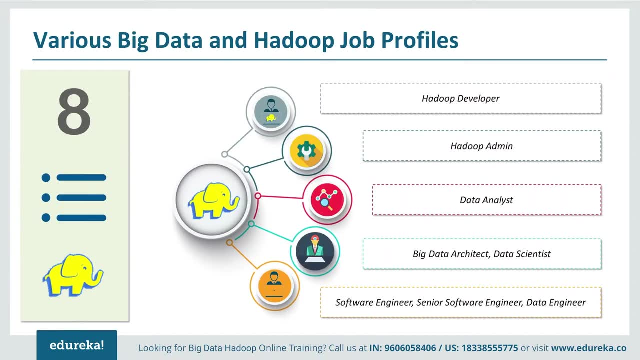 in the IT world. So if you start with big data, I'm very sure that you're going to have a bright future ahead. Reason number eight: the different big data and Hadoop job profiles. So there are various job profiles in big data and Hadoop Learning. big data and Hadoop doesn't mean that. 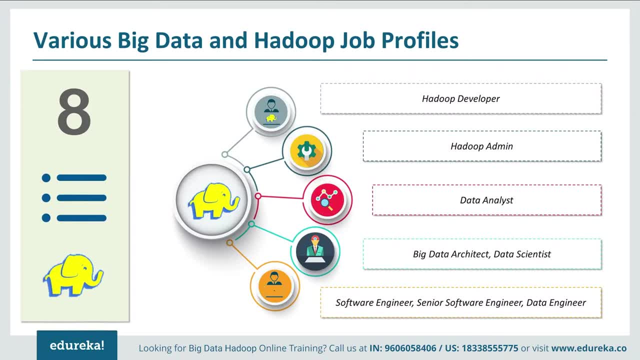 you'll be sticking on to just analytics. You can pursue any one of these job roles based on your professional backgrounds: You could be a Hadoop developer, a Hadoop admin, a data analyst, a big data architect or a data scientist, software engineer, senior software engineer, data engineer. 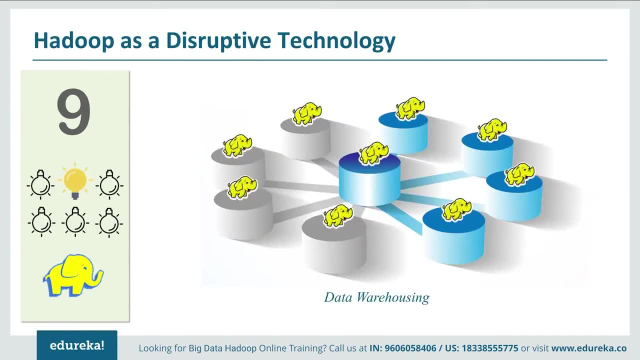 whatever seems more convenient for you. Reason number nine: Hadoop is a disruptive technology. When Hadoop came into the market, it completely disrupted the existing market and created a market of its own. Hadoop has proven itself as a better, more efficient option than that of traditional data warehousing systems in terms of cost. 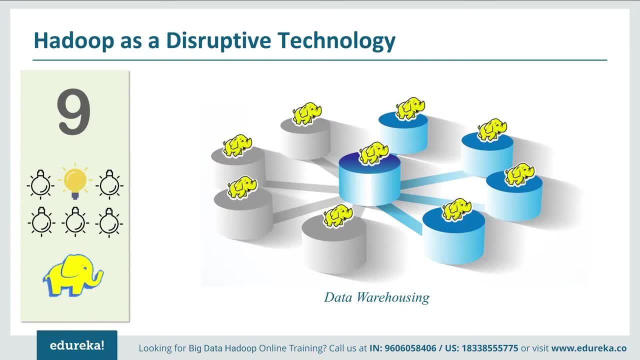 scalability, storage and performance over a variety of data sources. It can handle structured data, unstructured data and semi-structured data. In fact, Hadoop has revolutionized the way data is processed nowadays and has brought a drastic change in the field of data analytics. Besides, 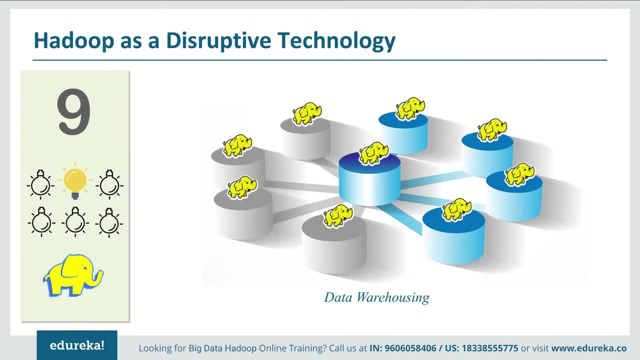 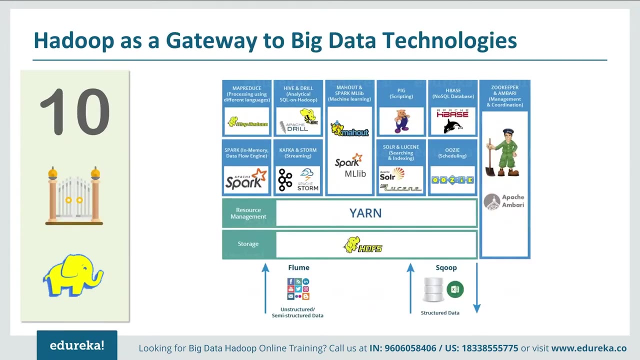 this Hadoop ecosystem is going through continuous experimentations and enhancements. In a nutshell, I would tell you that big data and Hadoop is taking out the world by storm and if you don't want to get affected, you have to ride with the tide. Reason number 10 and the most important one, Hadoop is.